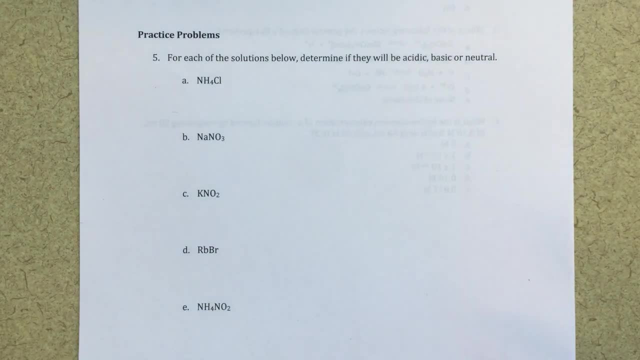 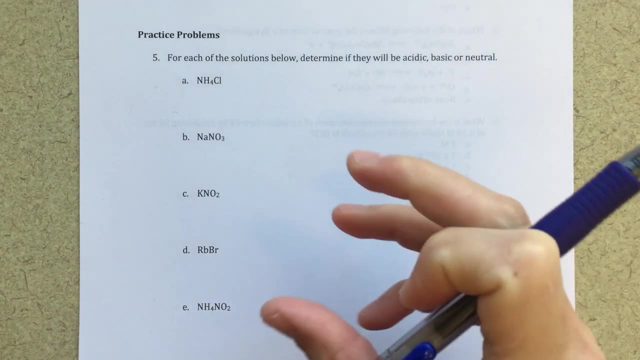 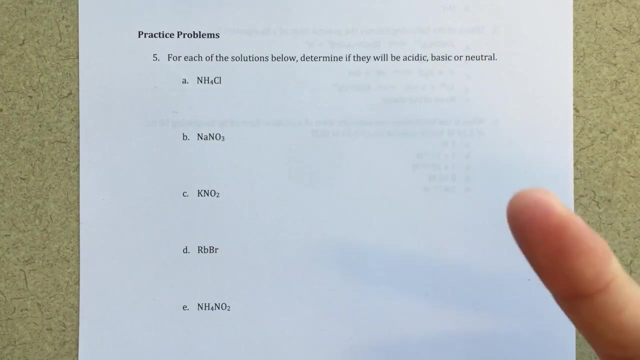 Alright, class. so this is the acid-based properties of salt, section 15.10. and this section we're gonna be talking about if these salts basically, once they dissociate, if they're gonna give an acidic basic or neutral solution, and I find that this is something that's really difficult for us to to predict. 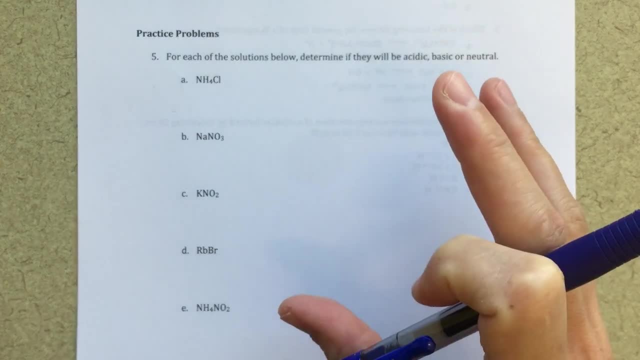 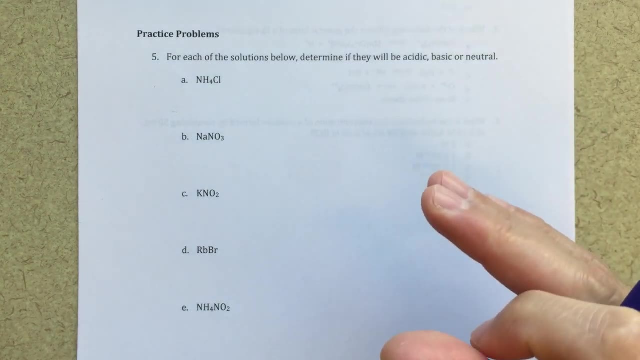 especially when we're starting out. so, for all of these, the first thing that we're gonna want to do- and you really have to sort of do this in a stepwise fashion. you have to be disciplined to say, okay, what's the first thing that I do, and then do that and then move on to the next steps to to solve the problem. 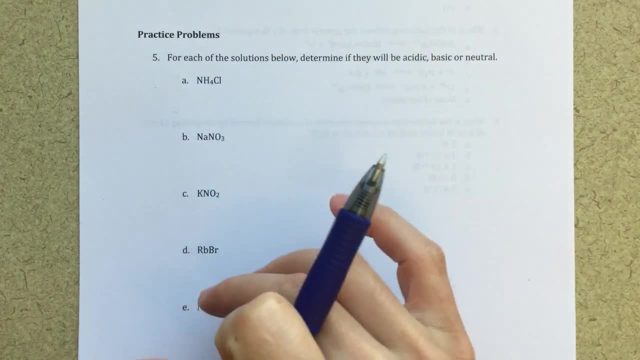 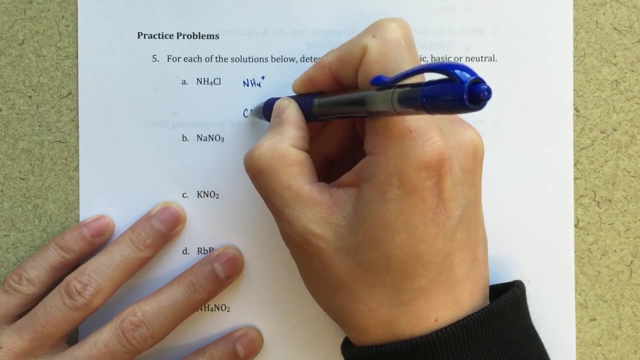 the first thing that we're gonna do is we're going to dissociate each of the salts. so when I see NH4Cl, really I'm seeing NH4 plus and then Cl minus, so I'm seeing both of those things right, because it's going to dissociate in. 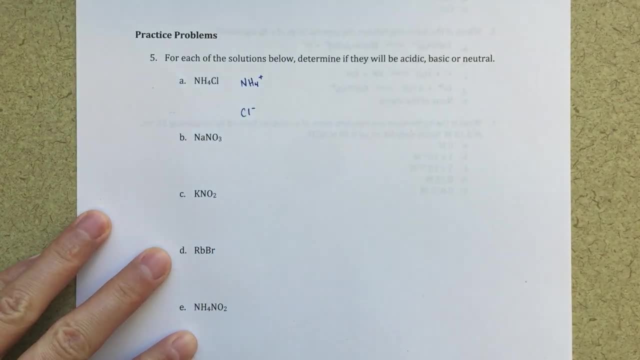 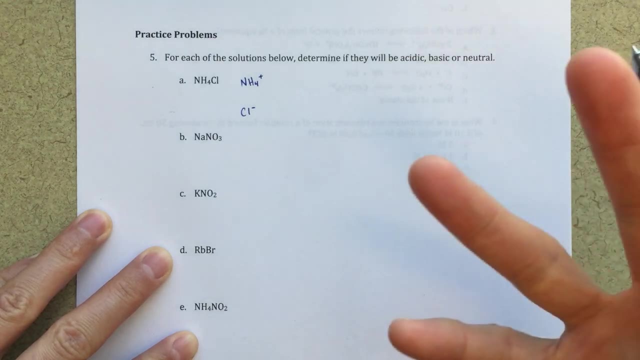 solution. all of these examples that we're giving you here. they're all going to dissociate into their respective ions, like it says, acid-based properties of salts. when I think of salt, I'm thinking of acid-based properties of salts and I'm thinking of acid-based properties of salts. when I think of salt, I'm thinking: 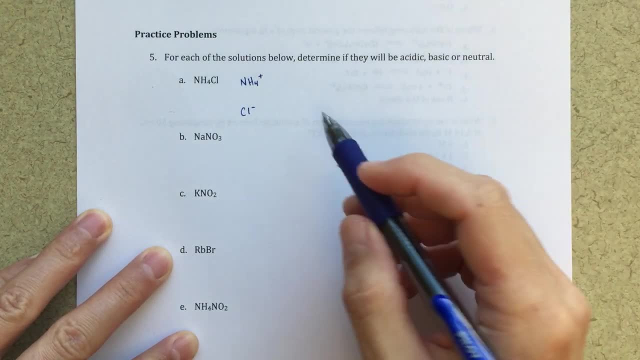 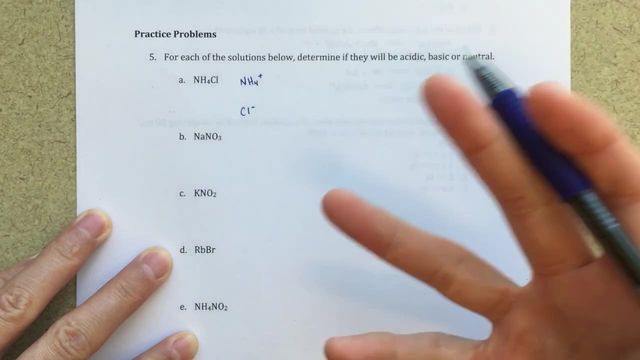 I should think of ions, right? The next thing I'm going to do is I'm going to consider the hydrolysis reaction. So what that means in maybe English means react it with water and see if anything happens. So when I say react it with water, I really just mean react it with water. 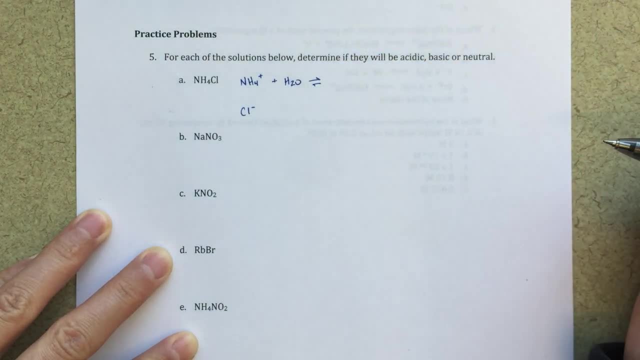 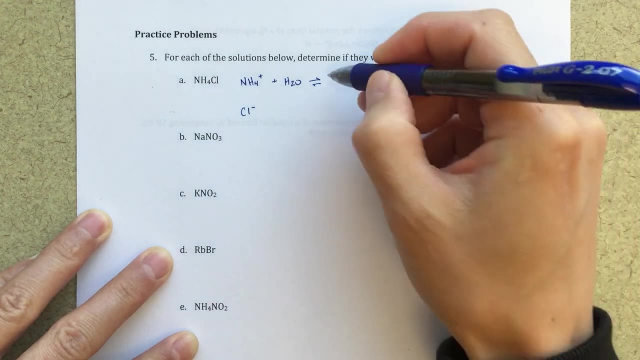 And then we're going to see if this reaction is going to be an equilibrium reaction or if it's not going to sort of go in one direction. And I can see this NH4+. It seems reasonable to me that we could end up with NH3 and H3O+ in this case. 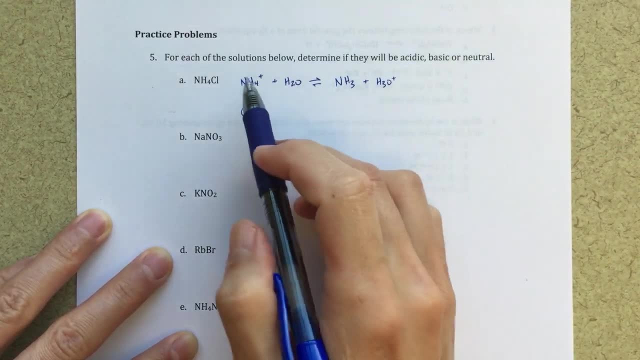 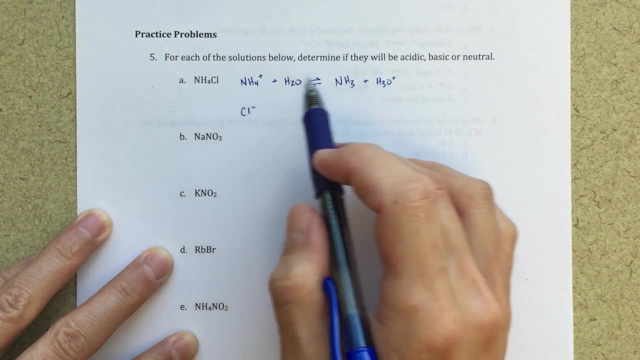 Now, in terms of predicting what's going to happen if you see a positive charge on this side, well, if you're going to do a reaction with water, then that means you're going to form H3O+. We want to have positives together, right? 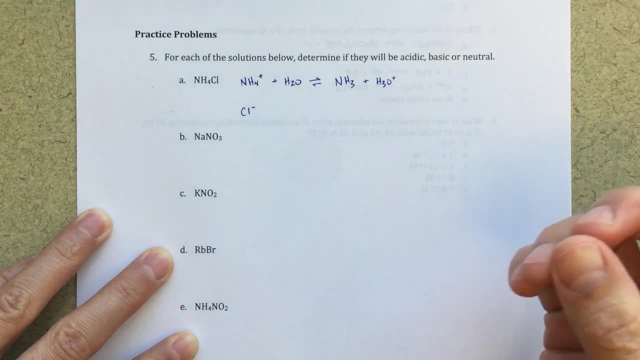 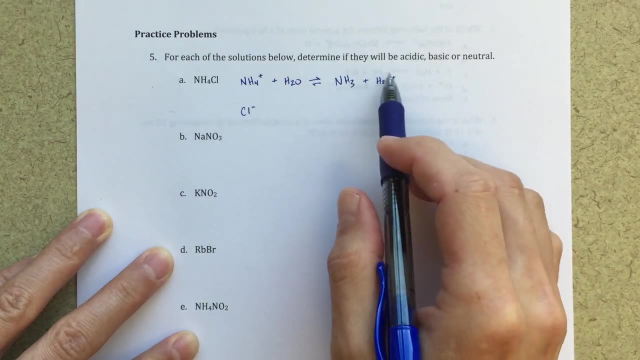 Charge balance. And then for the Cl- we'll see that we're going to want to have negatives together, So we'll see OH- in that case. So this would be the first reaction And we have to ask ourselves: is this a reaction? 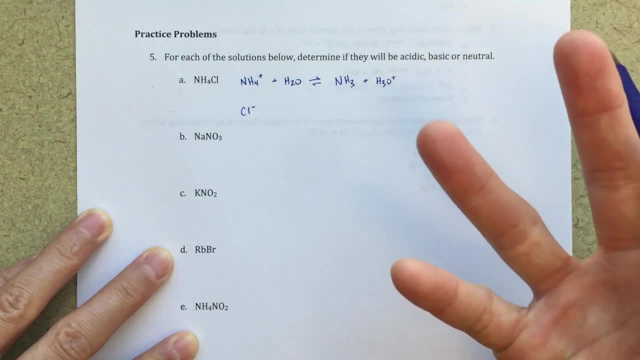 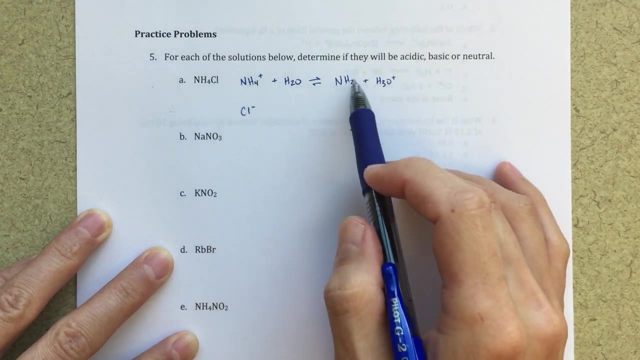 That could go appreciably to the right. Could this happen? essentially NH4+ plus water, giving us NH3 and H3O+? I see that this looks like a weak acid. This looks like a weak base. There's nothing that's sort of suggesting to me that this can't go to the right or go. 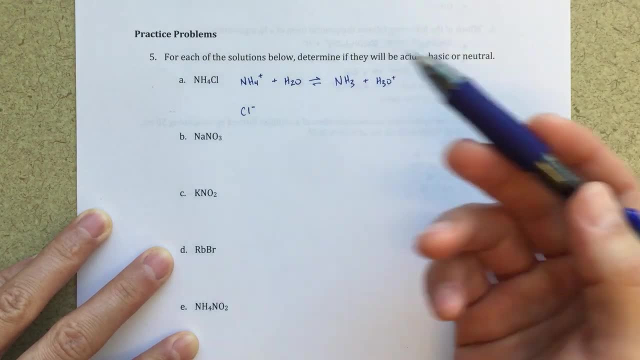 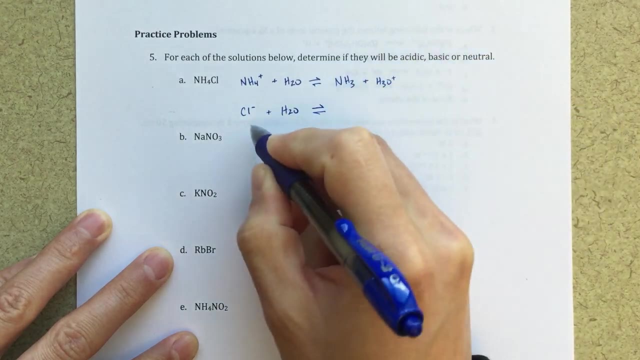 back to the left. So this seems like it could be an equilibrium And this seems very reasonable. Now let's consider Cl- So in this case, since we've got Cl-, the positive charge is going to be negative, So we're going to have a negative reaction. 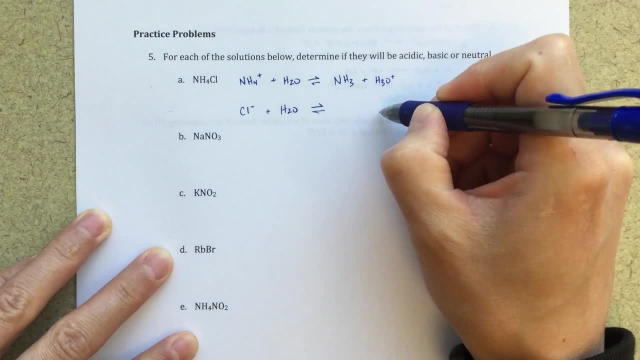 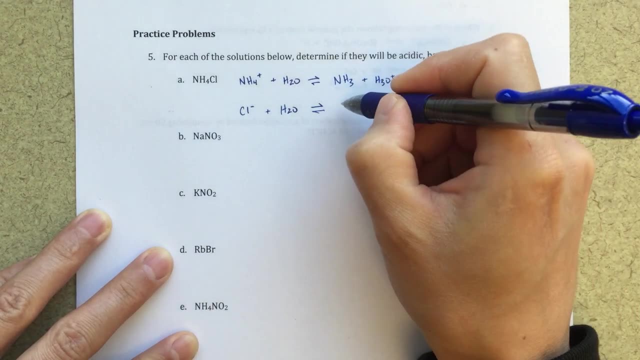 So we're going to have a negative reaction. So for the products essentially that I'm going to be looking for, one's going to be OH-. so, since I see this, minus here, minus here, And then the other product- if I took OH- from H2O is going to be HCl. 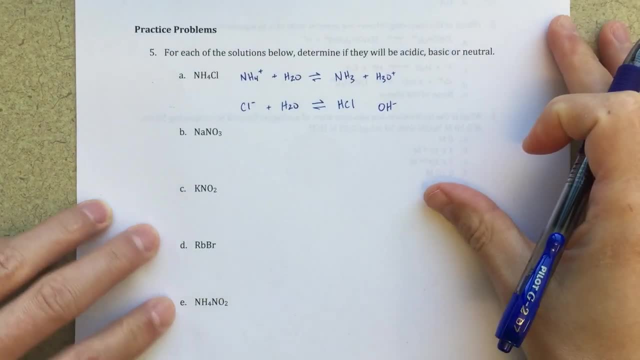 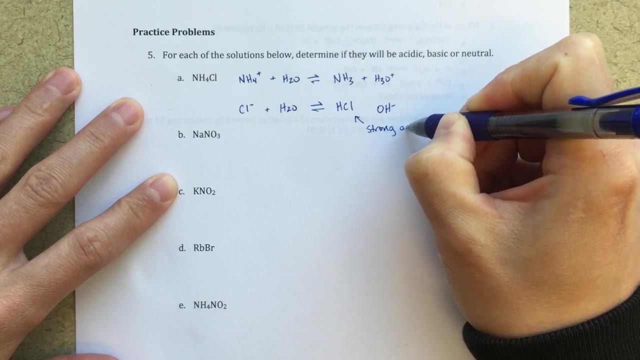 And when I see that HCl I should have sort of warning bells going off in my head, because the HCl I need to recognize as a strong acid And that strong acid is not going to be stable in solution, It's not going to be ever – you know, if you've got H-floating around, you've got H-. 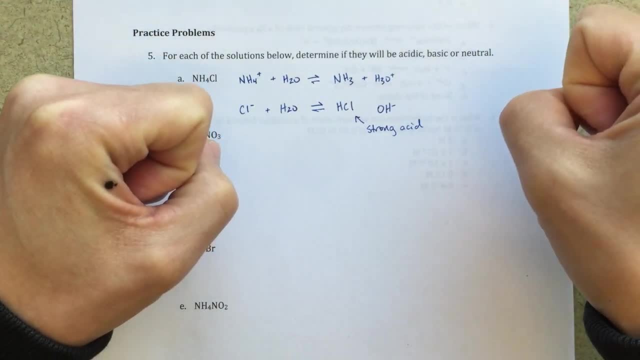 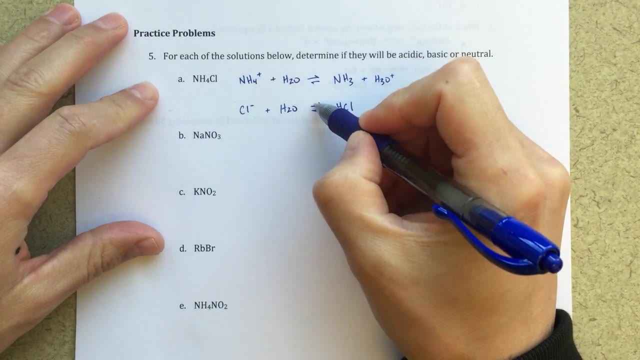 floating around. you've got Cl- floating around, right, and they're separate in the solution. they're never going to come together and form HCl. That's not going to happen, right? So this reaction here, it is not going to do the top reaction, It's not going to move to the right. 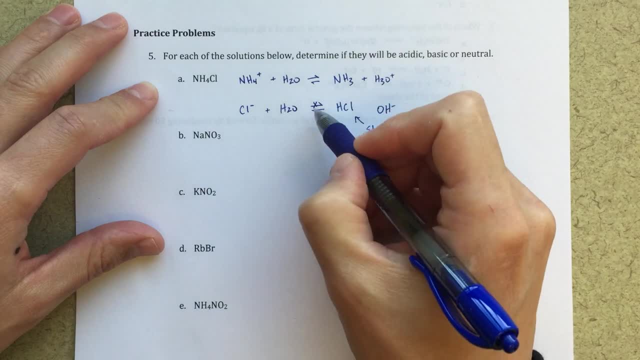 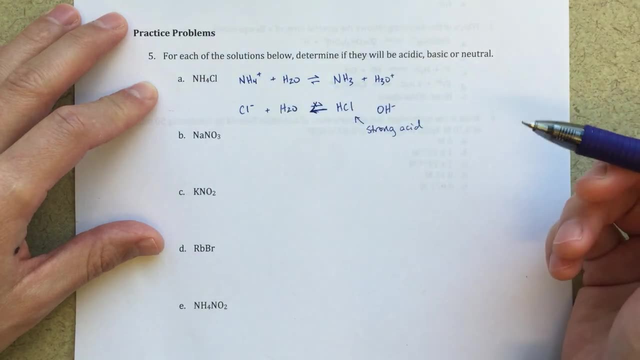 at all. Zero percent, right, If you put HCl in solution, we often draw reaction arrows going in one direction. just going this direction would only be able to go to the left. It's not going to be able to go to the right. Okay, Now we need to decide. well, what does that? 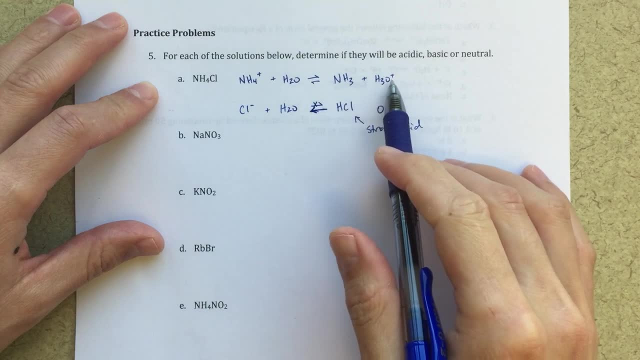 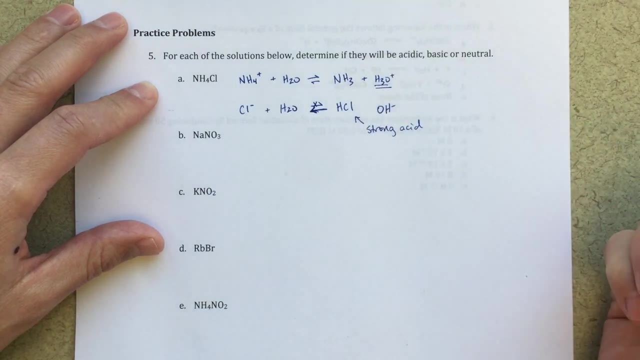 mean for this overall solution: NH3 Plus plus H3O Plus- essentially what we're doing. if I have NH4 Plus and Cl-, I'm going to be putting a little extra H3O Plus into my solution, but I'm not putting any extra OH- into the solution, right, Since there's no extra OH-. 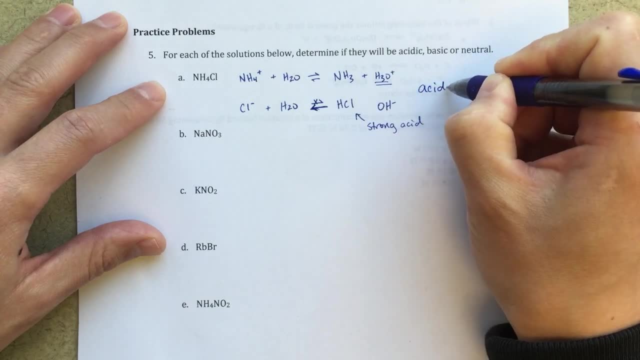 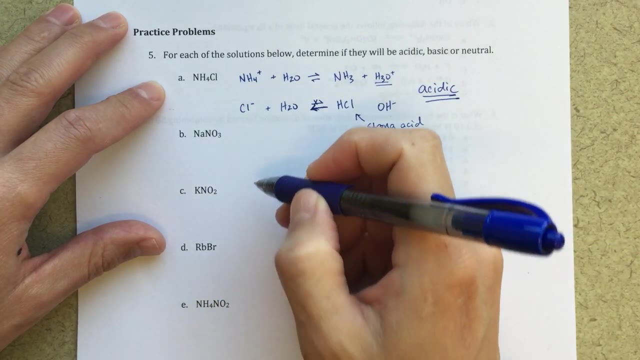 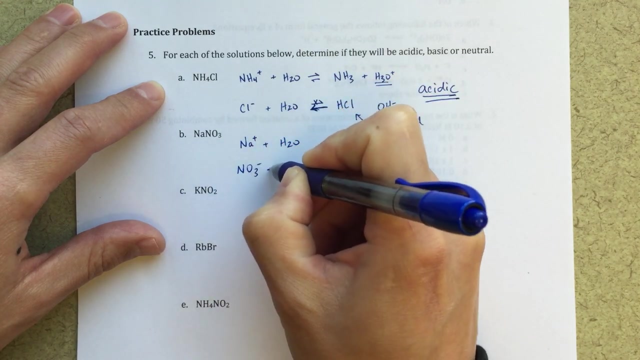 in the solution. overall, this will be slightly acidic, And that's based off of this H3O Plus solution that we put into the solution. So let's do some more examples and see if we can catch on here. Again, I'm going to dissociate into ions. 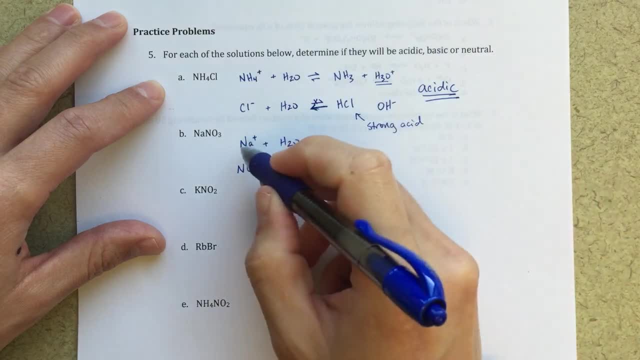 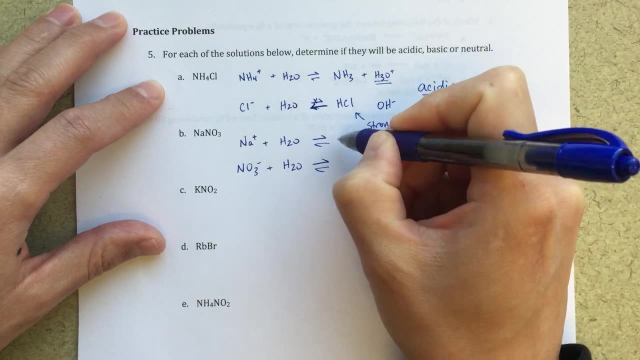 and then consider the hydrolysis reactions. So in this case, Na plus again. since it's plus, I'm going to be expecting to form H3O plus as one of my products, And then whatever's left over will be sodium hydroxide. 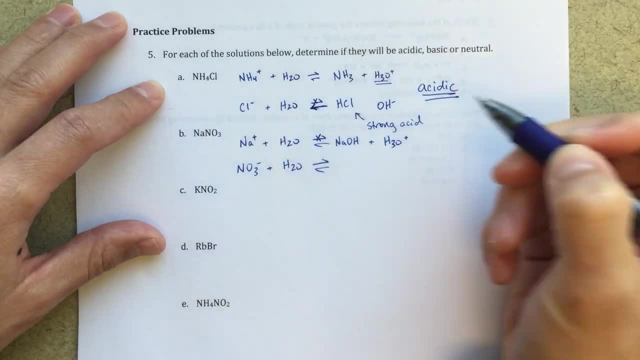 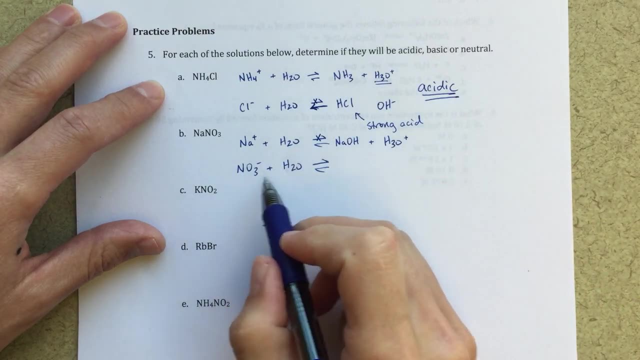 That's a strong base. Since that's a strong base, this reaction is not going to go any way to the right at all. It would only go back to the left. So we're not going to be putting any H3O plus in. 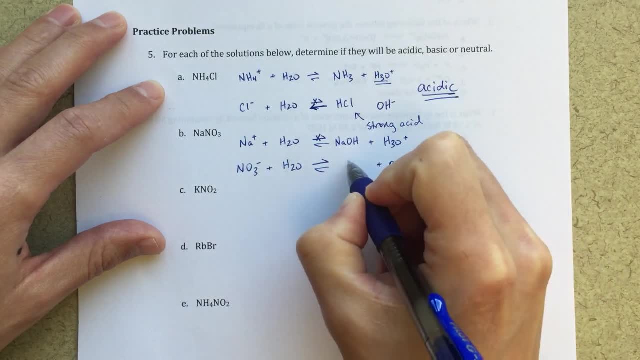 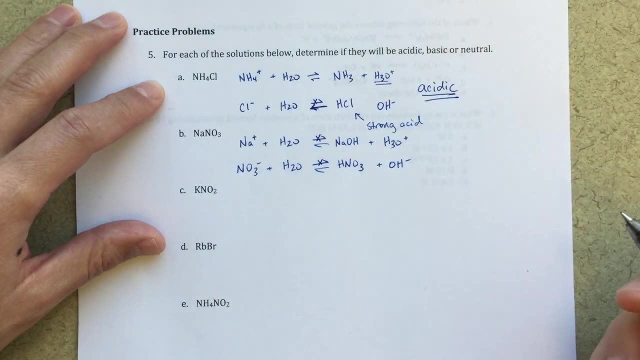 Again, we'll do the same thing here: OH minus plus. Now in this case it would be HNO3. Again, strong acid. So again, this reaction is not going to go appreciably to the right at all. 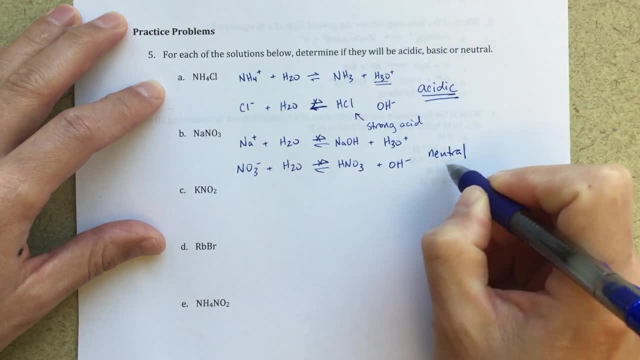 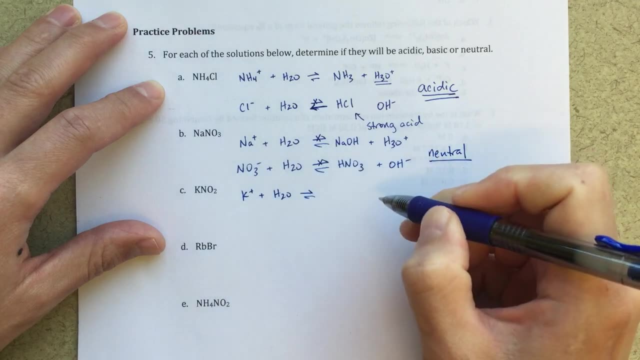 So again, this one will be neutral KNO3.. So again it's the same process: H2O. Here we're going to be forming again H3O plus, And then what's going to be left over? 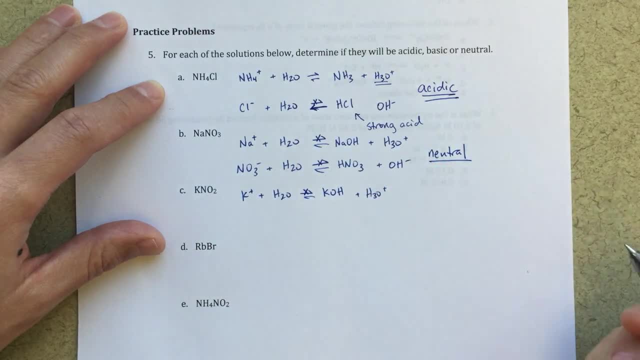 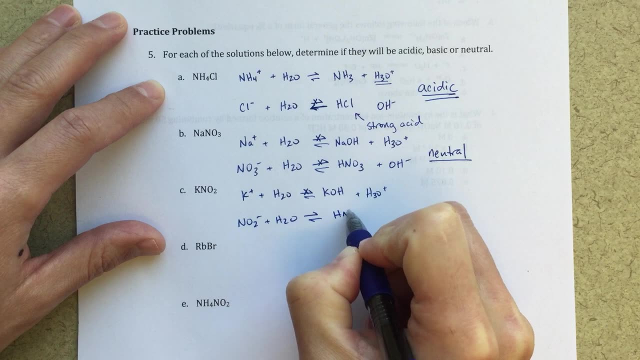 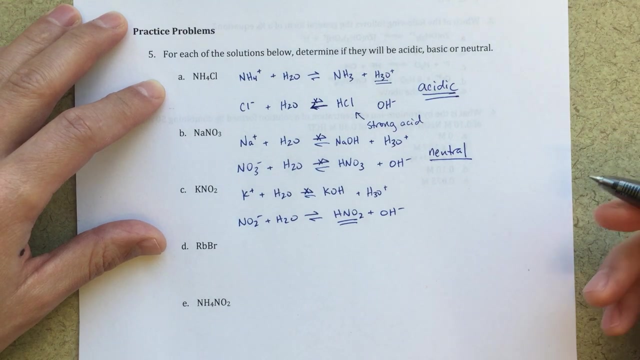 KOH strong base, So this reaction is not going to happen. And then NO2 minus plus H2O, We're going to get HNO2, NOH minus, And here we've got a weak acid, This HNO2, that is a weak acid. 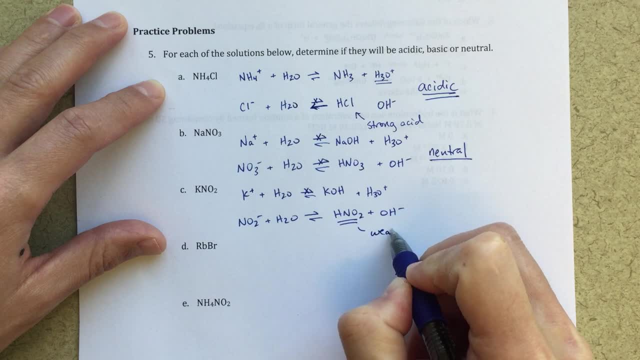 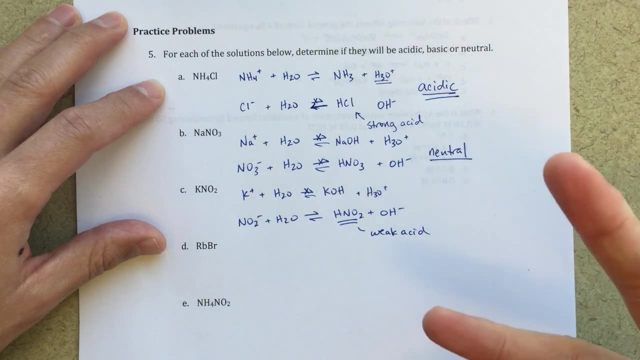 Therefore, this reaction could go. So we'll call this a weak acid. So this reaction can go A little bit to the right. The significance of it being a weak acid is simply that it is stable in the solution. Since it's stable in the solution, 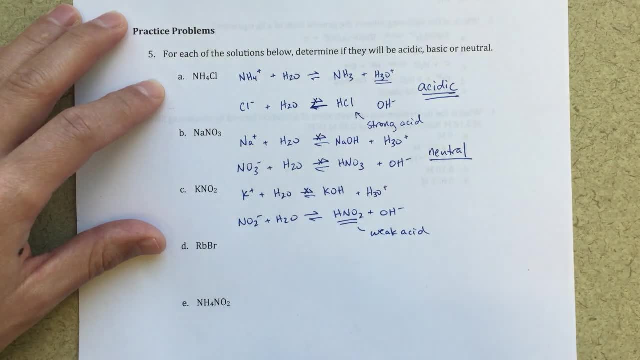 this reaction, this equilibrium, it can go a little bit to the right. That's sort of the whole point here. So this one's going to be basic. And it's basic because I'm putting a little bit more OH minus. It's a little confusing, right. 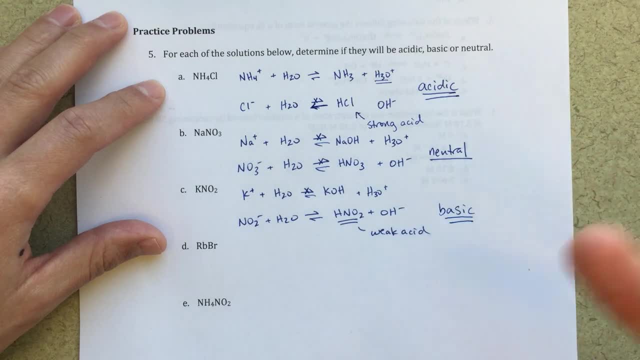 You're forming a weak acid And therefore it's going to be a little bit more basic, Like what. That doesn't make sense, But it does make sense because as we form that little bit of weak acid, we're also forming OH minus. 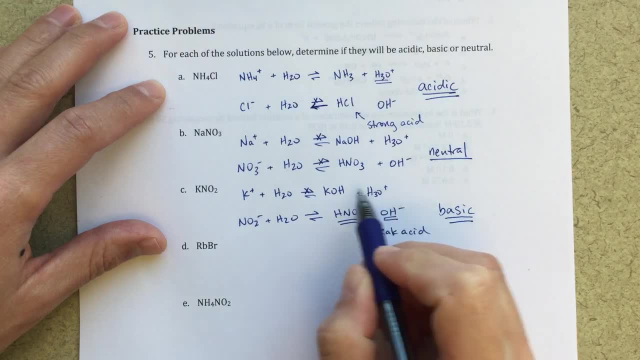 So this OH minus here, that's what's telling us that this KNO2 solution is going to be, overall, a little bit basic, right, The K plus this is just going to be a spectator, It's not going to do anything. 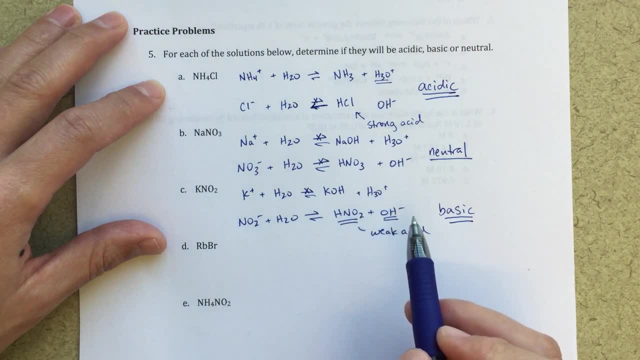 It's not going to form KOH, It's not going to therefore form a little bit of H3O plus. So we're going to have K plus NO2 minus, And because this NO2 minus can do this hydrolysis reaction, 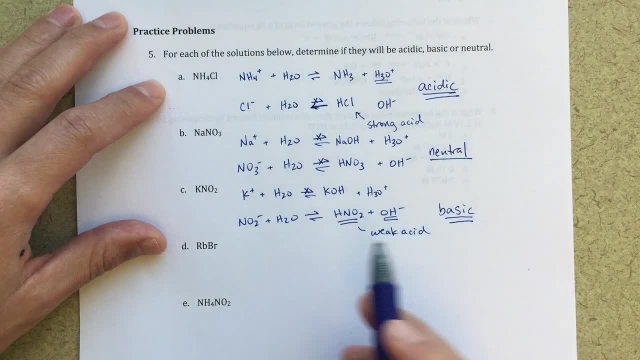 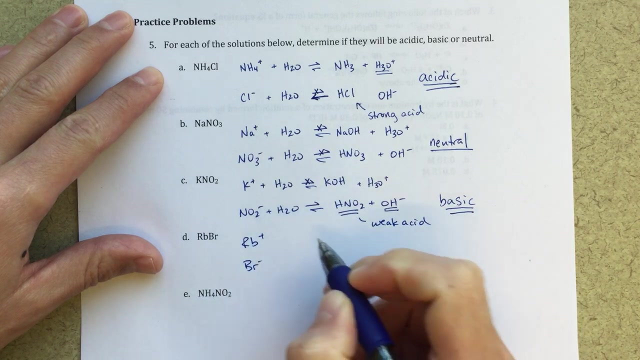 well, it's going to be putting a little bit of OH minus into the solution. Therefore we have an overall basic solution. So the logical progression there is a little bit complicated, right, But hopefully it will make sense. Now the next one: RB plus BR minus hydrolysis reaction. 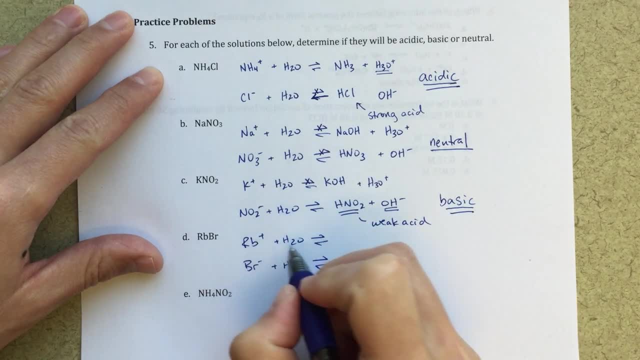 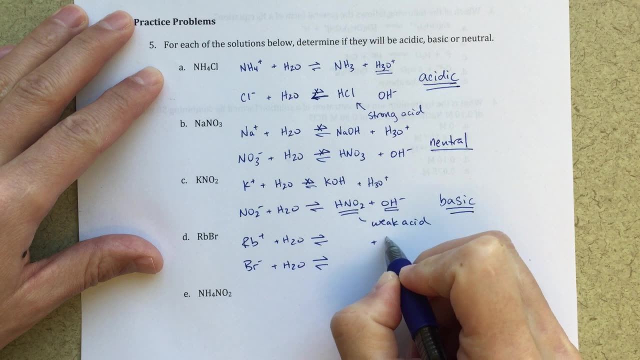 hydrolysis reaction. Now again, since I see the plus, sometimes you're looking at this, you're like what products are going to be formed? I don't really know right. But again, if you see the positive here, 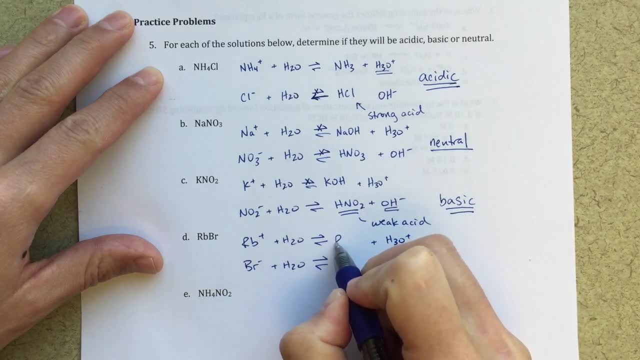 that means we're going to have H3O plus And then what's left over, Rubidium OH. So this is a strong base And we need to be able to recognize that right from our just looking at the periodic table. 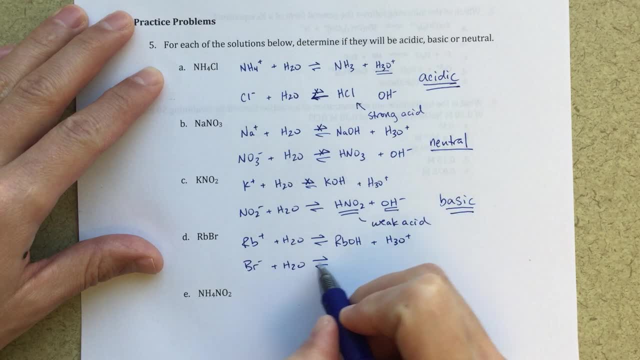 we should be able to figure out that that is a strong base. And then BR minus would be HBR plus OH minus. Again, the OH minus is the hint there. And then HBR is the strong acid. This one's going to be neutral. 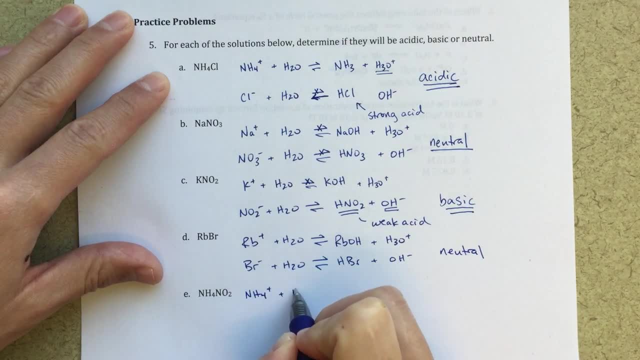 Finally, we've got NH4 plus. We already know that that's going to work, that that's going to give us NH3, which is a weak base, plus H3O plus And NO2, again, earlier we saw that that is also. 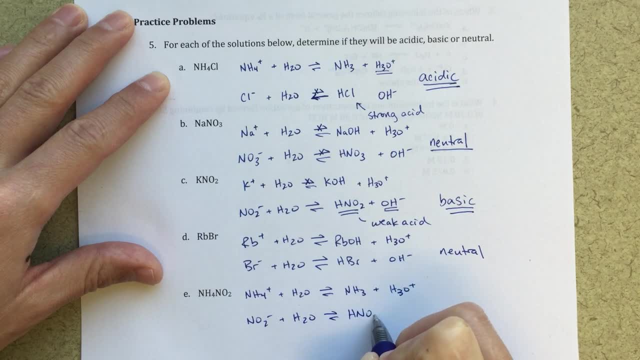 going to undergo that hydrolysis reaction to give us HNO2.. That's a weak acid plus OH minus. So now we need to figure out well which one of these is going to go to the right to a greater extent. 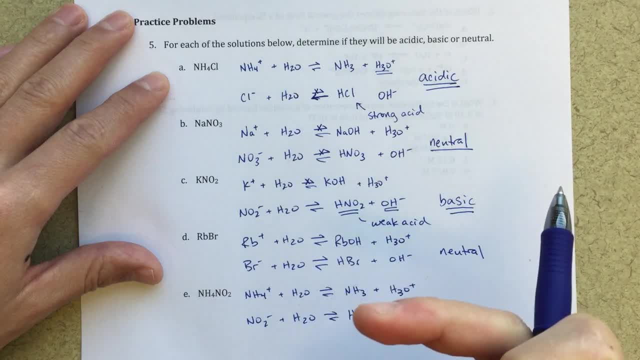 We're going to have NH4 plus and NO2 in an equal amount, because it's a salt. We would expect a one-to-one ratio there. So then, which one of these is going to go to the right to a greater extent? So what we're going to do is we're going to compare. 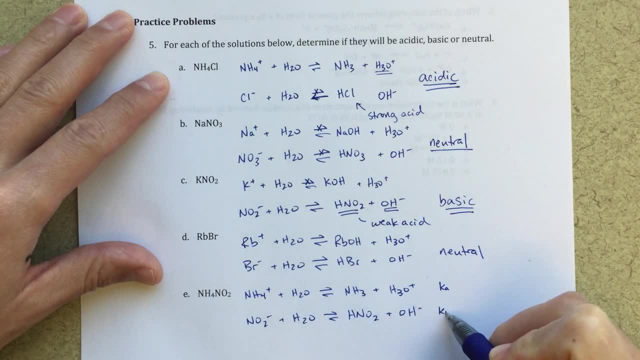 This is going to be a Ka That follows the general form of a Ka, And then we'll compare that to the value of this Kb That follows the general form of Kb. So here we've got 5.62 times 10 to the minus 10th. 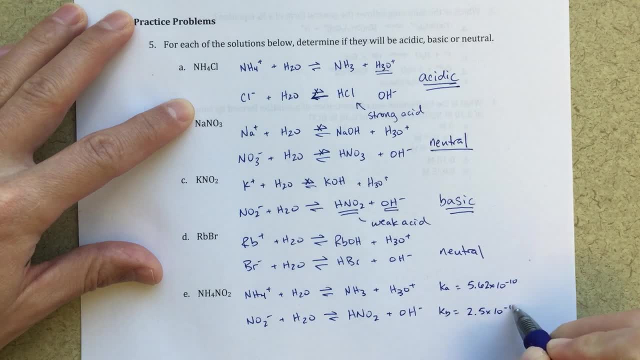 And here we've got 2.5 times 10 to the minus 11th. So this is a large base. This is a larger Kb, very, very small obviously, But this larger Kb- slightly larger Kb- is going to mean that there's slightly more H3O plus.